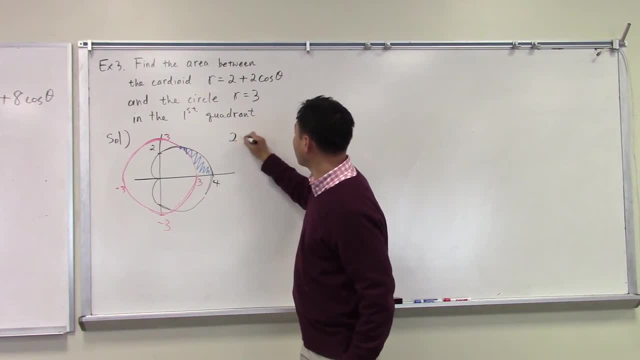 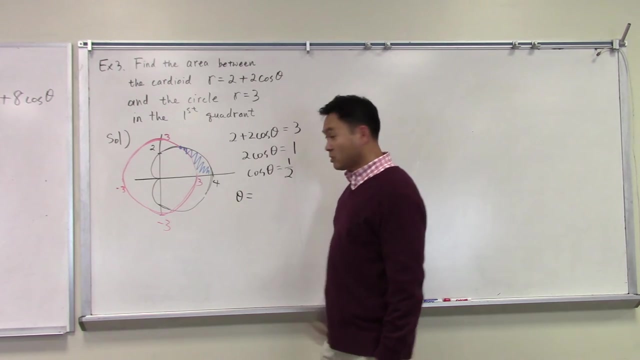 r is two plus two cosine theta r is equal to three. sets them equal to each other. Two cosine theta is equal to one Cosine theta is equal to one half. At what angle does cosine become one half? Sixty degrees, And in terms of radius this is pi over 3.. 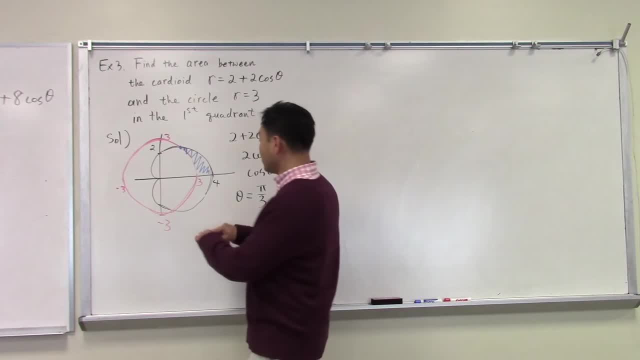 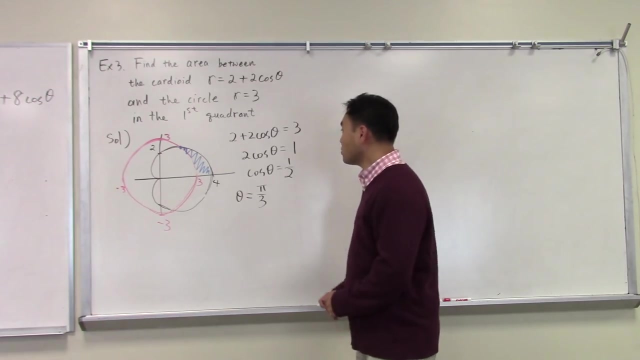 So you know that The rays that hit this region start from theta equal to 0 until when it passes through this point, which is pi over 3.. And in order to find the area enclosed, you have to use polar coordinate integration, double integrals. 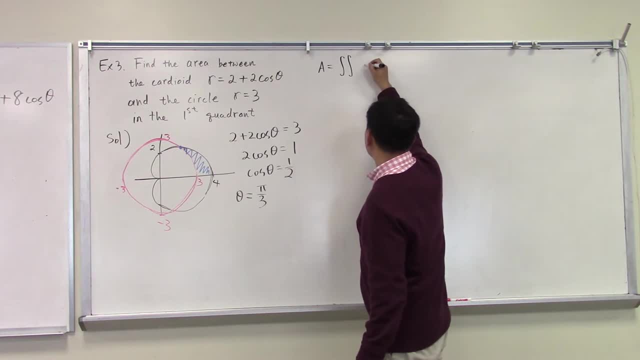 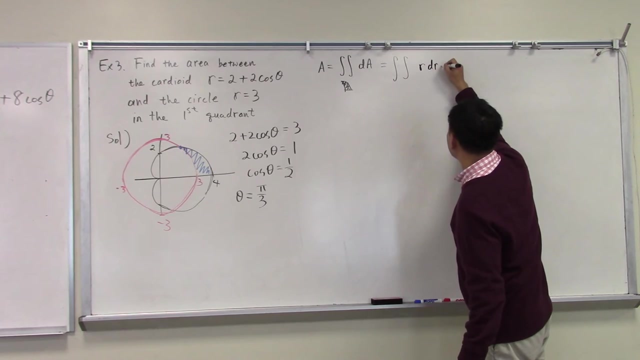 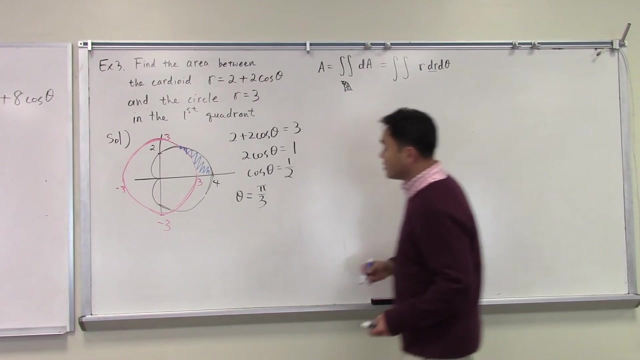 and polar coordinates, Just like that. you have to do dA over this domain that we just drew And whenever you write dA in polar coordinates, remember it's always r, dr, d theta, And since we have dr inside, that means we're trying to paint this region in radial direction. 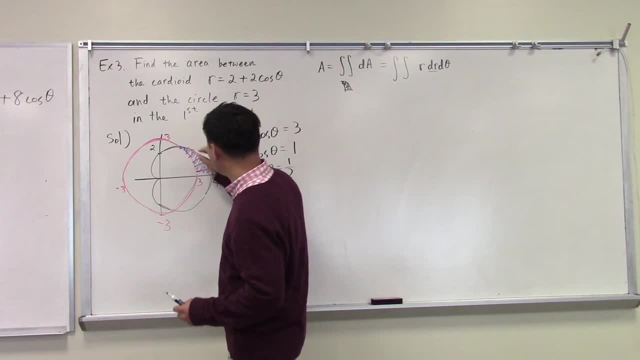 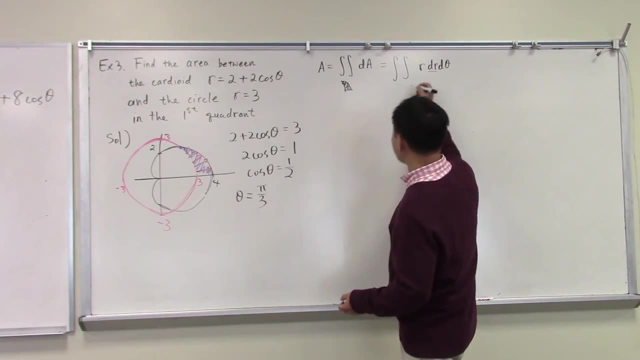 So we're trying to paint this region in radial direction like that, where you begin at this curve and then you end at that curve. So where do you begin? What's the equation for this curve? inside, r equals to 3, right. 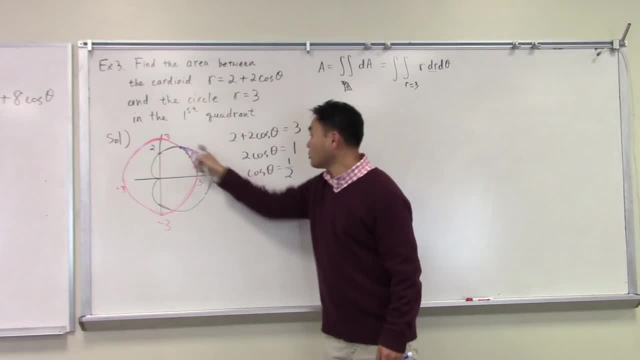 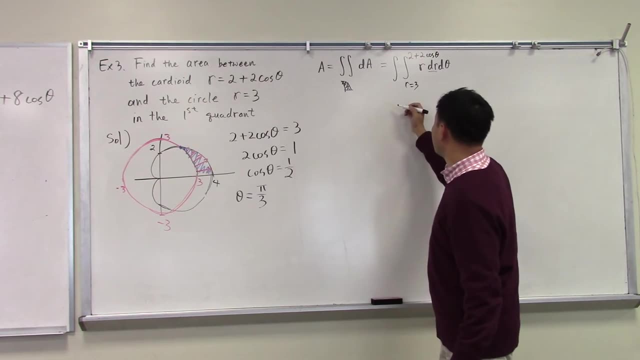 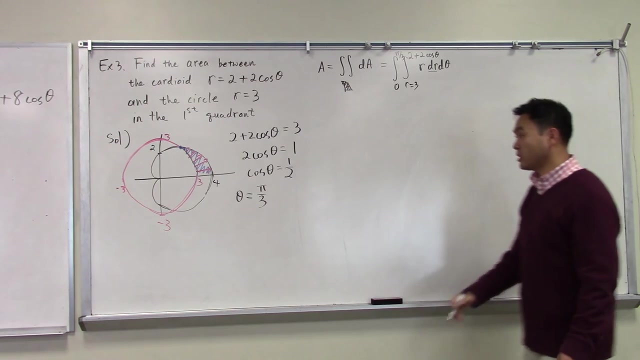 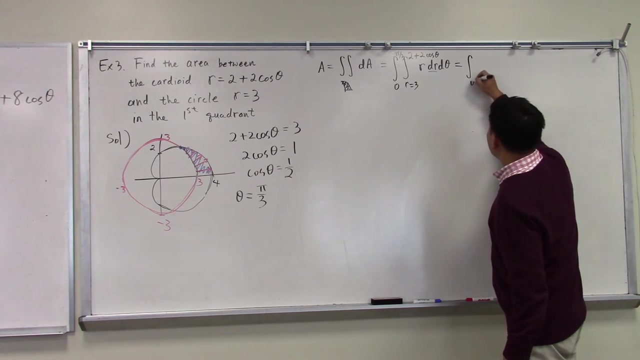 r equals to 3.. Where do you end? The outside curve has the equation given here, which is 2 plus 2 cosine theta, And then theta starts from 0 and ends at pi over 3, as we just have calculated. Now to actually calculate this, it's quite messy. 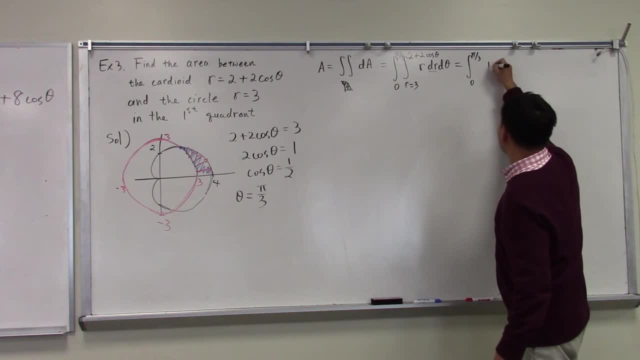 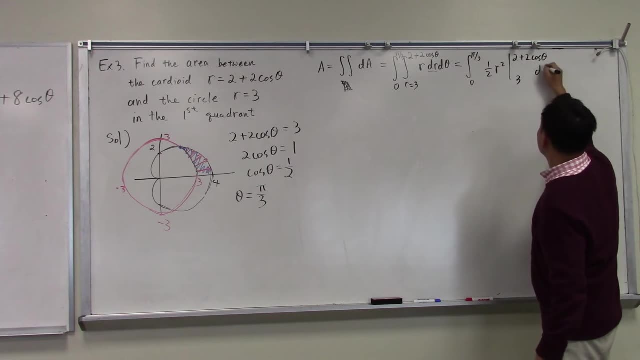 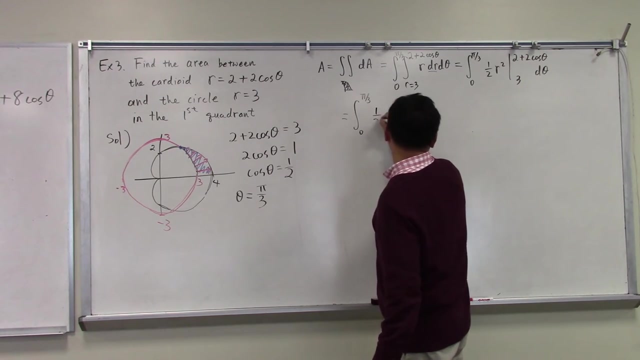 But let's try to do this. r if you integrate, that's 1 half r squared. You have to plug in 2 plus 2 cosine theta and 3 inside r, So you end up with 1 half 2 plus 2 cosine theta squared. 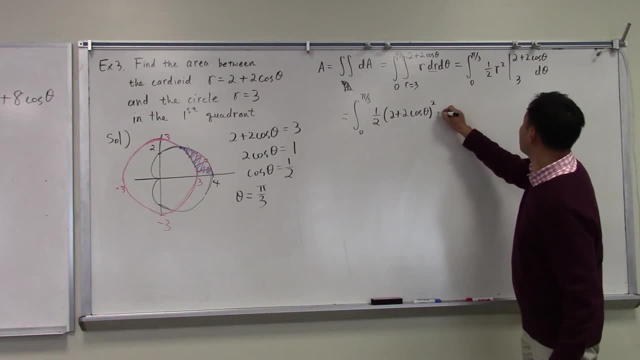 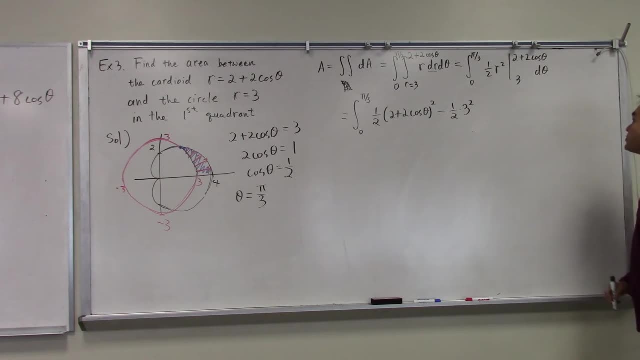 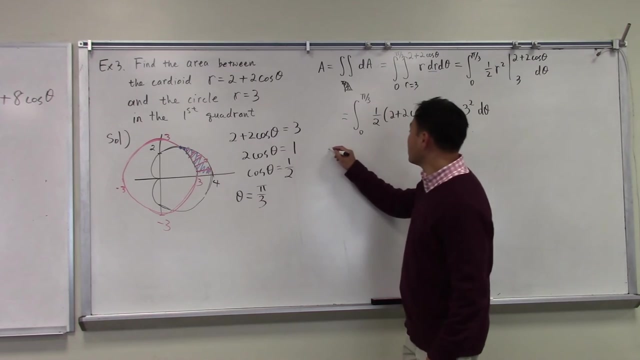 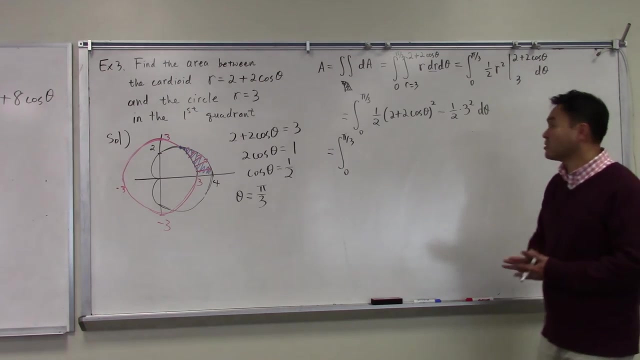 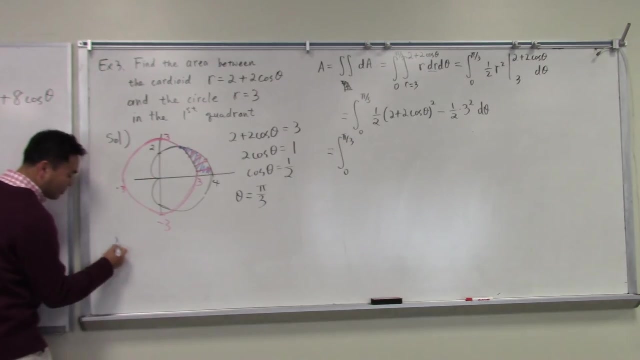 OK, OK, OK, OK, OK, Minus 1, half times 3 squared. You have to plug these in and you subtract If you expand this square by FOILing or using the formula. I think everyone knows this formula: a plus b squared. 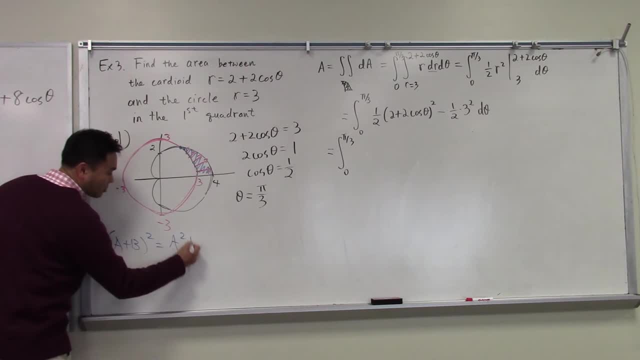 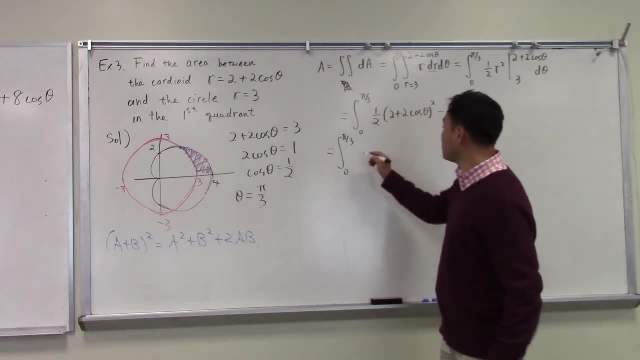 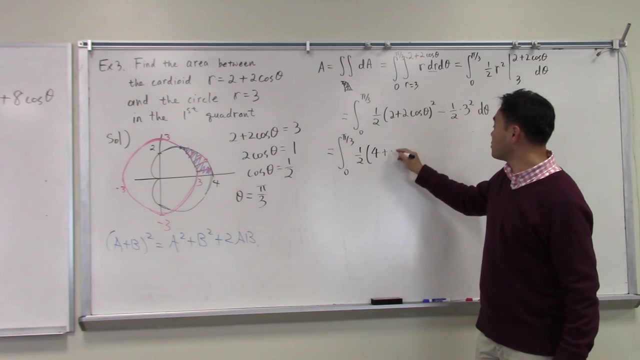 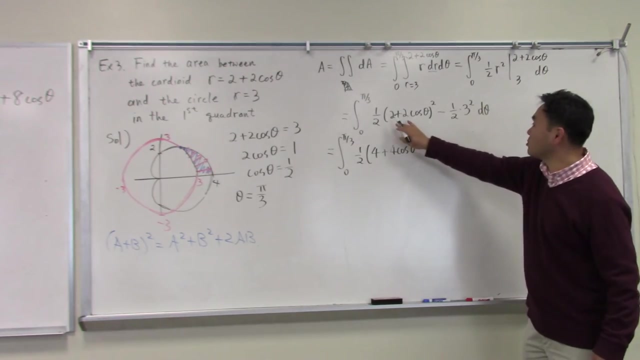 is equal to a squared plus b squared plus 2ab. it says I'm supposed to be doing square the first according to that formula, which is 4, square the second, which is 4 cosine squared theta, and you have to double the product, double of the product, right? So you do. 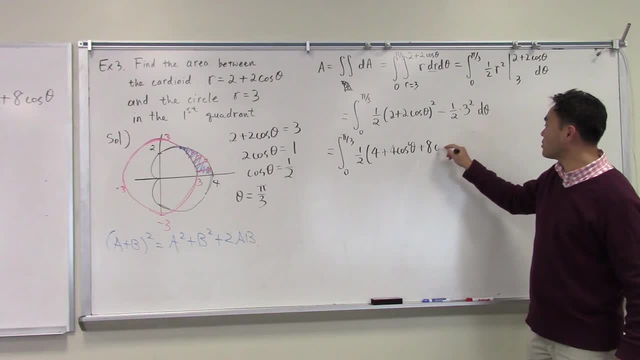 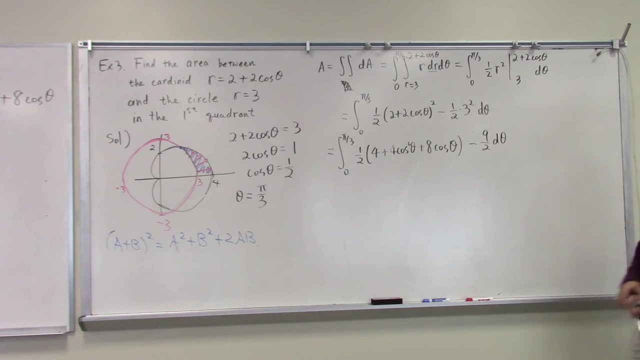 twice of the product, which is 8 cosine theta. This is what you get if you expanded this, if you use FOIL, And then this is 9 over 2 e theta. Okay, 4, you don't have any trouble integrating. 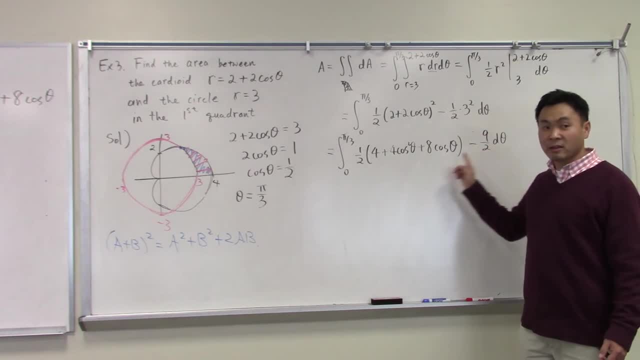 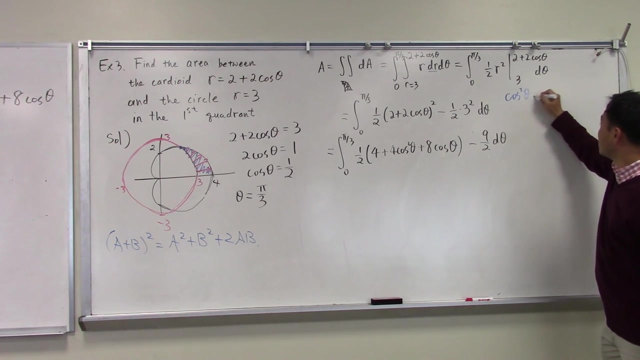 cosine theta, there's no trouble integrating. The only thing that will be a little hard to integrate is this cosine squared. To integrate this cosine squared, you need to use this formula that we discussed a moment ago: cosine squared- theta is 1 plus cosine 2- theta over 2.. Okay, so this is what we will do. 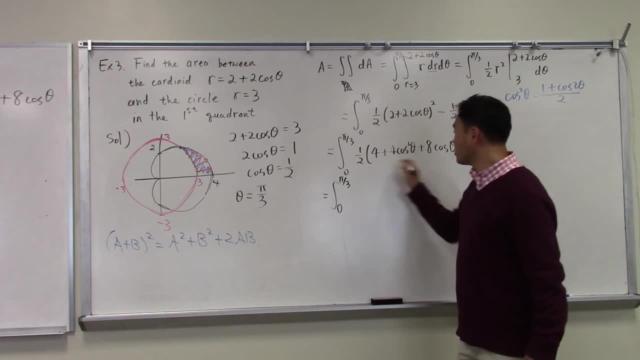 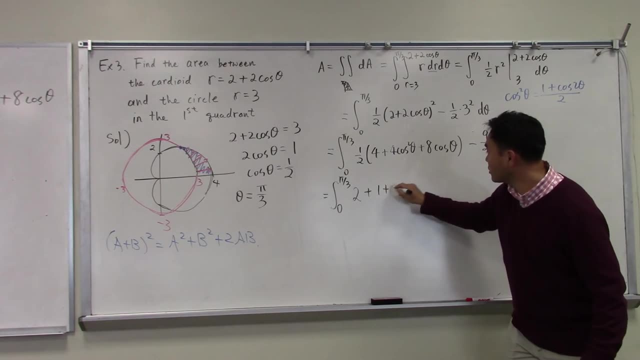 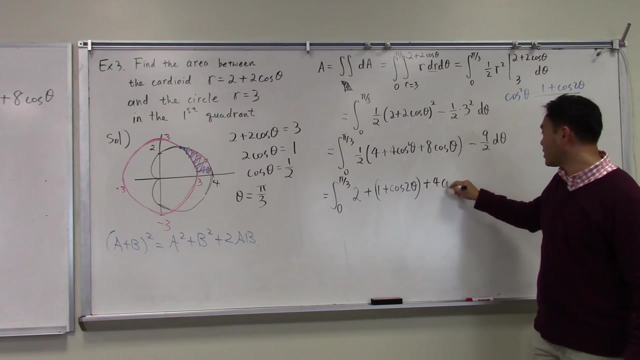 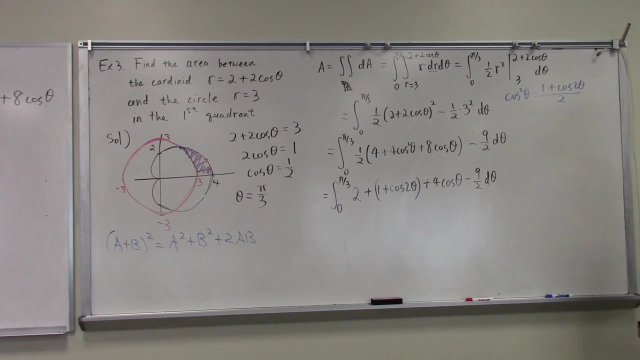 Multiply 1 half through, so it's 2, plus 2 cosine squared theta. but 2 cosine squared theta is 1 plus cosine 2. theta 1 half times 8. cosine theta is 4. cosine theta minus 9 over 2. e theta Okay, 2 plus 1 is 3, minus 9 over 2,. 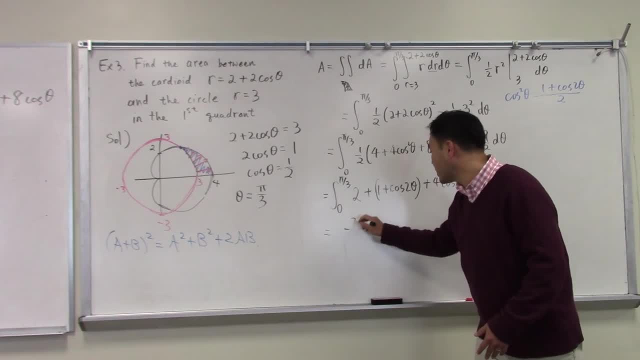 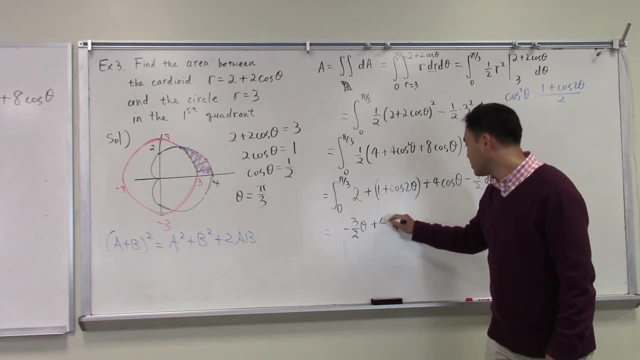 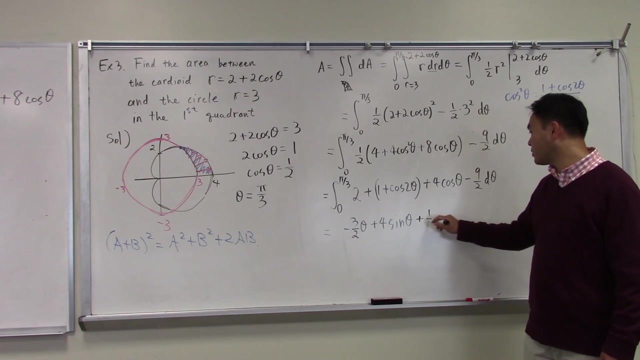 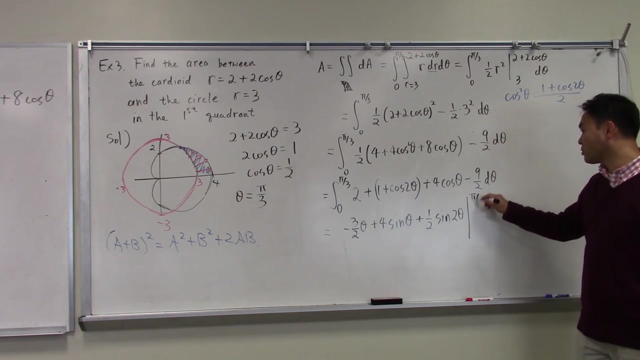 that's negative 3 over 2.. If you integrate negative 3 over 2, you get negative 3 over 2 theta. If you integrate cosine, you get sine, And if you integrate cosine 2 theta you get 1 half sine 2 theta And you have to plug in the end points pi over 3 and 0..